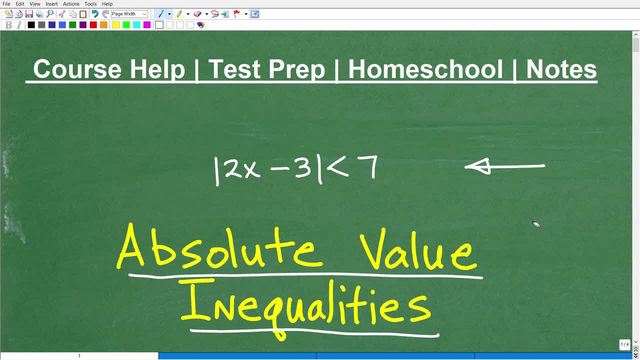 because a lot of students will study and learn how to solve absolute value equations And then when they look at an absolute value inequality, they'll do the same techniques or same procedure to solve an absolute value inequality. They'll be using the absolute value equation procedure, And you know. 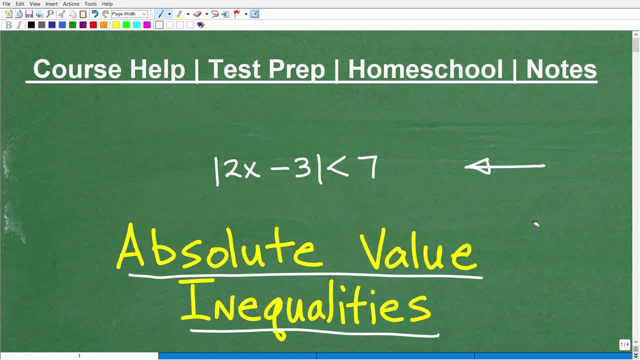 this is a very common mistake that I see with math students, So you don't want to confuse the two because they, you know, are completely different. But we're going to get into how to deal with absolute value inequalities in just one second. Actually, if you know how to do this problem, go ahead and do this. 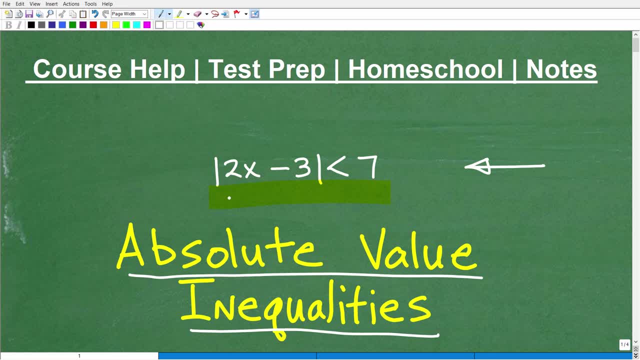 real quick and put your answer in the comment section. Now we do want to have a graph to this, the respective graph as well. You won't obviously be able to put that into the comment section, but you can put in an inequality statement that represents the. 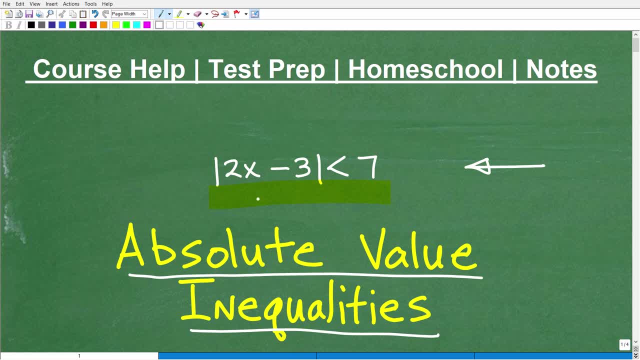 solution to this inequality. So if you can do this stuff, go ahead and put your answer into the comment section, But we're going to get into this in just one second. But first let me quickly introduce myself. My name is John. I'm the founder of Tablet Class Math. I'm also a middle and high school math teacher. 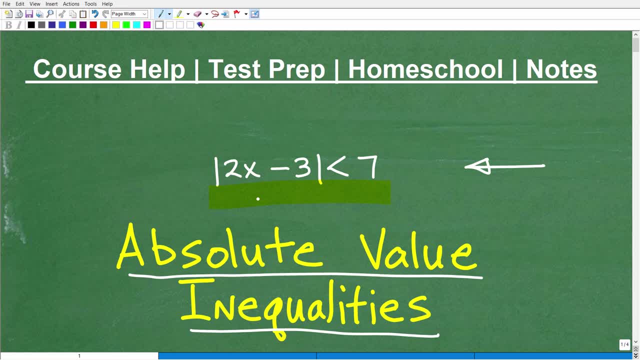 I'm going to leave a link to my math help program in the description of this video. But if you are frustrated in mathematics, maybe you know you've. math has just not been your your topic and you just have a lot of anxiety about it. 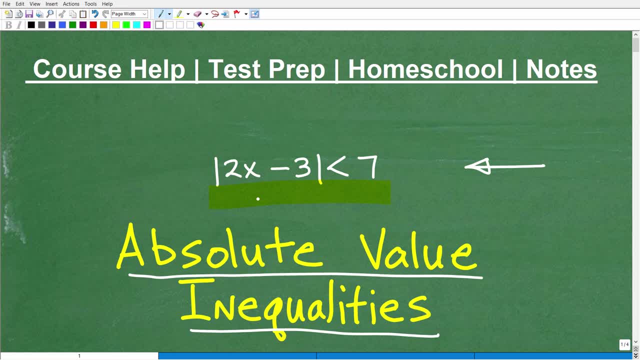 Maybe you don't feel like you're getting enough instruction at school or maybe you don't connect with your teachers Teaching style. Well listen, I've been teaching math for decades and I really pride myself in breaking all these concepts down into really bite sized. 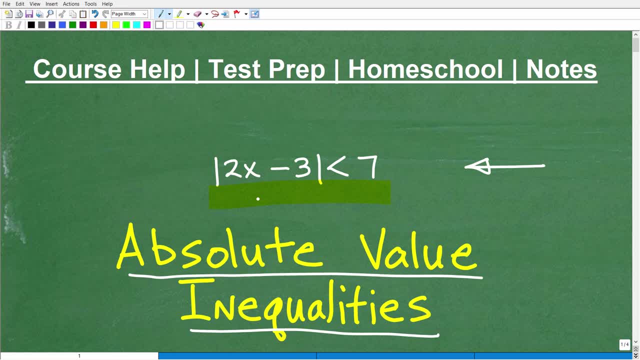 super clear and understandable kind of concepts so anyone can be successful in math. So if you're at the middle school, high school, even college level in terms of mathematics, I can help you succeed in your respective math courses. Now, if you're studying for any test that has a math section on it- I'm talking about things like the GED, SAT, ACT, GRE, GMAT, ASVAB, ACCUPLACER, CLEP exam, teacher's certificate- 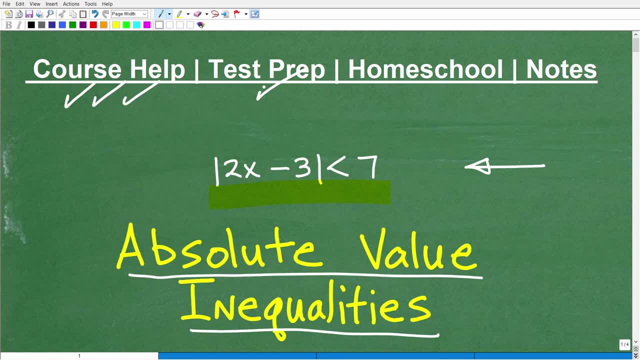 education exam, nursing school entrance exam, I can go on and on and on, but you get the idea I can help you prepare and pass those exams If you homeschool have an outstanding very comprehensive homeschool math program that you might want to check out. 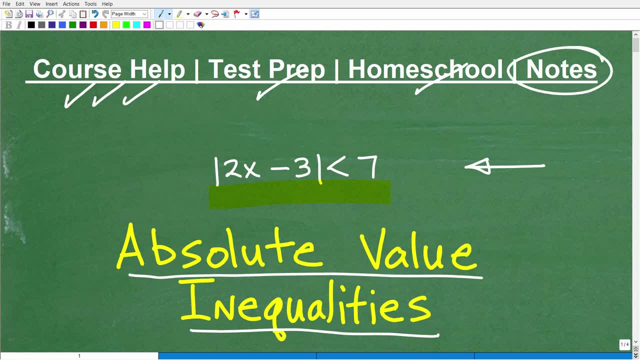 And if you don't have any math notes, don't panic. I'm going to leave links to my math notes in the description of this video, But I'm going to tell you right now: if you want a great grade in math and your math course, you've got to have great math notes. 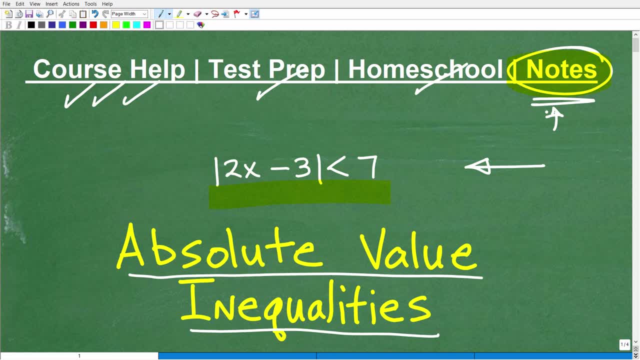 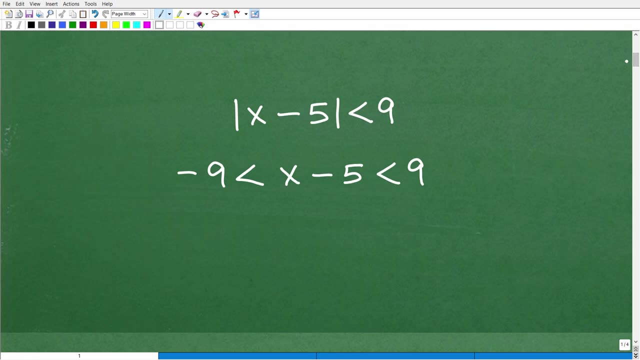 This is non-negotiable. OK, So start improving your notes and you'll see magic start happening. All right, So let's get into absolute value inequalities again. I'm going to be doing this problem here in a second, but let's get into a more basic problem first. 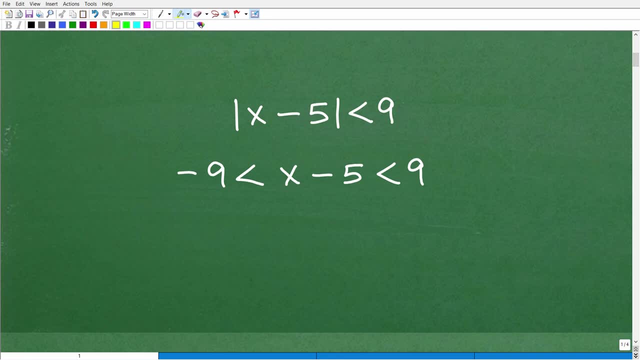 OK, All right. So here, basically, This is the setup to do an absolute value inequality. Now, let's just notice this is a less than OK. So we have a variety of different absolute value Inequality symbols we can have along with absolute value. 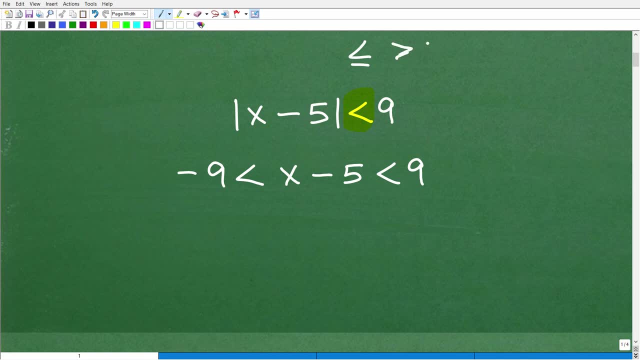 So you can have the less than, less than equal to greater than and greater than equal to. So, basically, the procedure is effectively the same, But you've got to be very, very careful when you're doing this. Now I will say, as a prerequisite, you need to understand how to solve compound inequalities. 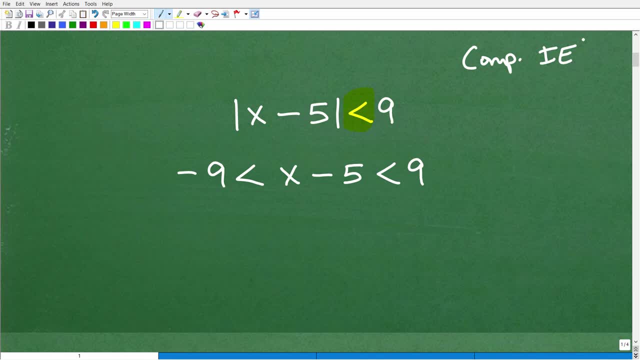 OK. So if you're not familiar with solving linear inequalities or compound inequalities, then you're going to- you're going to want to go back and review that, But you'll probably be able to- To pick up how to solve these if you forgot as I go through the steps. 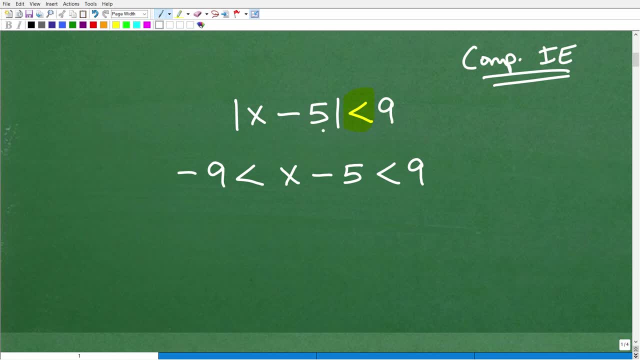 OK. So in this basic problem here, OK, Of course, we have the absolute value function and an inequality symbol less than OK. So we have: this is less than nine. So what is the setup? Well, we can't do anything with this set up right as it is right now. 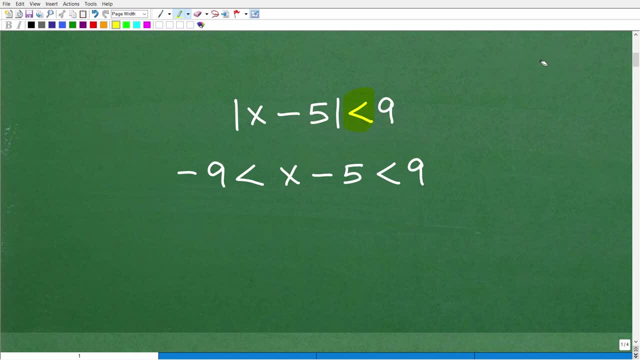 Well, actually we can, OK, But I guess what I'm getting at is, in order to solve an absolute value inequality, we have to have only the absolute value function on the left hand side and a number on the right hand side, just like this. 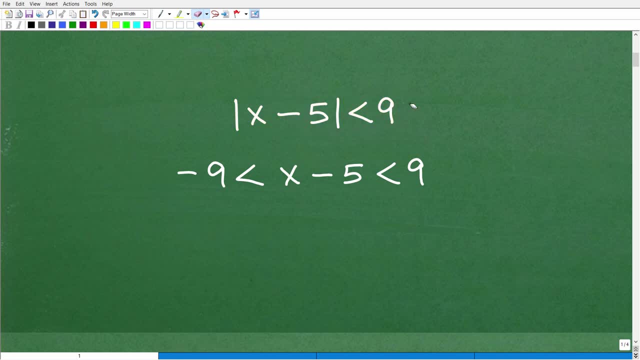 So this is already set up nicely for us right now. So I didn't mean to confuse you, But what I'm trying to say- not every problem is going to be set up all nice and beautiful like this, But we're going to start with a nice, easy problem, All right. So notice, I have my less than symbol. 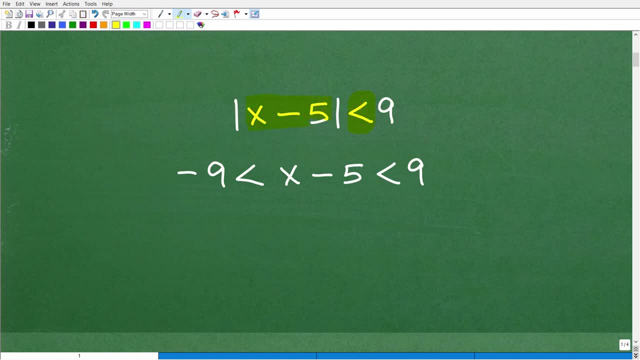 So what you're going to do is you're going to take what's inside the absolute value function, And in this case it's X minus five. We're going to put this in the middle. OK, Then we're going to take this number, whatever number this is. 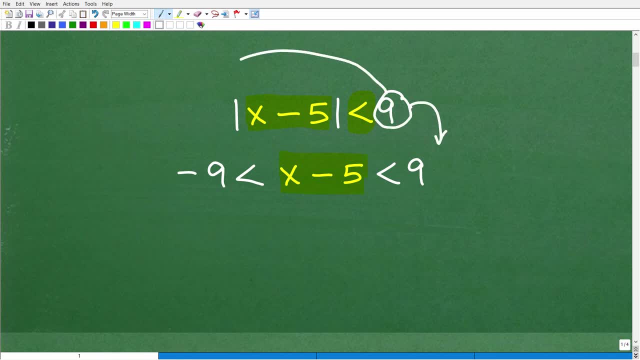 OK, We're going to put this over here and we're going to put the opposite or the negative of that number over here, And we're going to keep the same inequality symbol: X minus five. We're going to surround that by the less than here and a less than here. 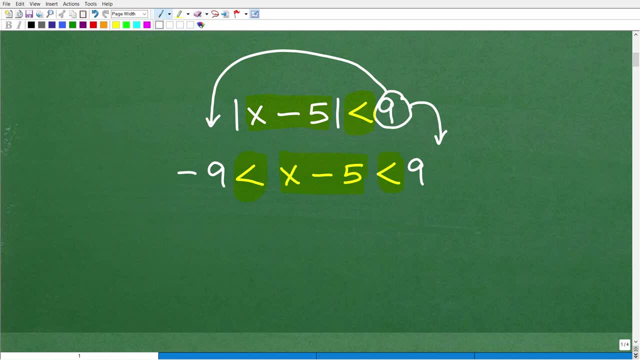 So let's make sure you understand this, because this is how we're going to do all these problems. So let me actually take this from a different point of view. So the first step is you're going to take whatever is inside the absolute value function. 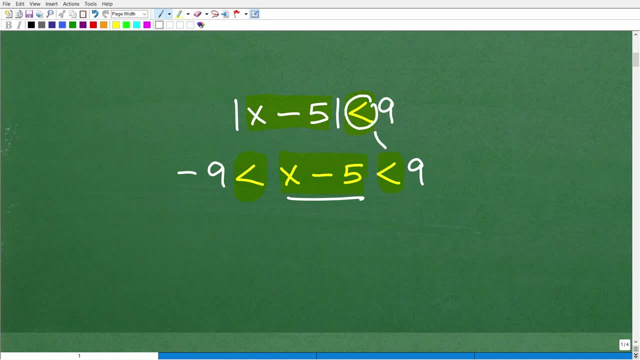 We're going to put that in the middle, and then we're going to surround that by this inequality symbol. It's less than here, And then we're going to put a less than there, And then we're going to drop this number. whatever it is, we're going to put it right there. 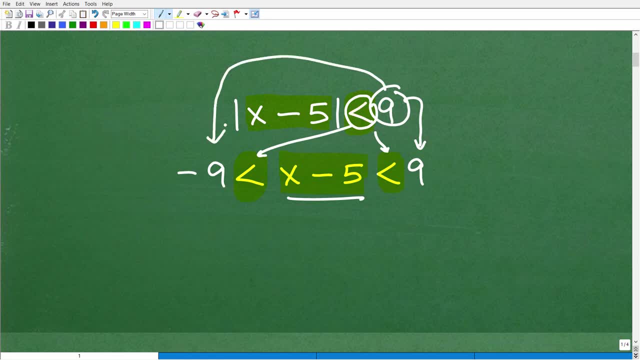 And then we're going to take the negative of that number and put it right there, OK. So as long as you understand what I just showed you right here, OK, You're going to be able to solve any absolute value inequality Now. 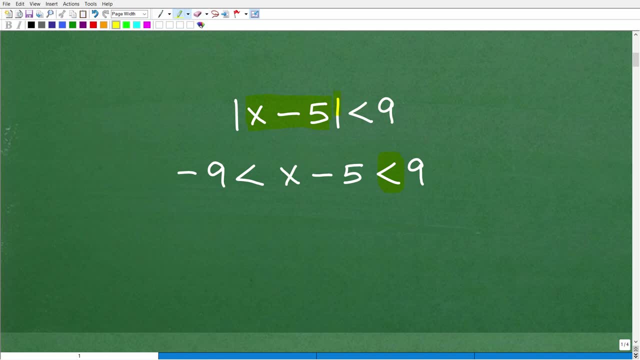 You can't do this, set up and until and unless you have only your absolute value function on the left hand side and a number on the right hand side- And not every problem is going to be like that- You're going to run into more challenging absolute value problems, something like this: 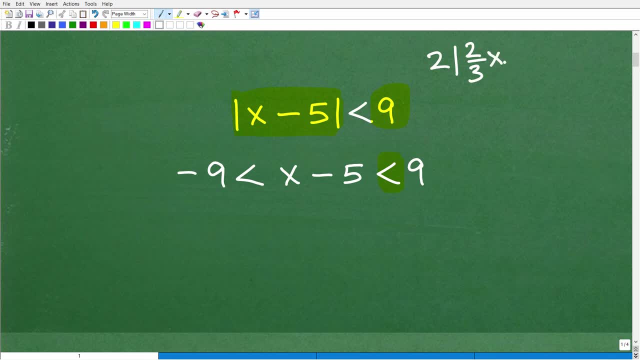 The absolute value two times absolute, two thirds times X minus, let's say five, And then we might have minus one. Let me move this down here. I just want to show you an example of something that's going to require more steps greater than equal to. 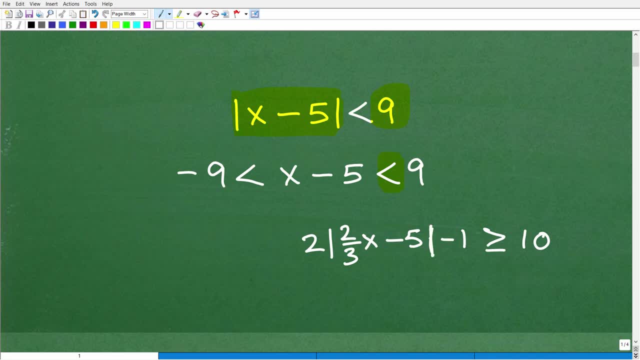 Let's say ten. OK, So here, this isn't. this absolute value portion right here is not isolated all by itself on the left hand side. So we have some cleanup to do in order to get it to this step. But again, I want to start off with what we do. once we have an absolute value inequality written, where it's just absolute value, function and number. 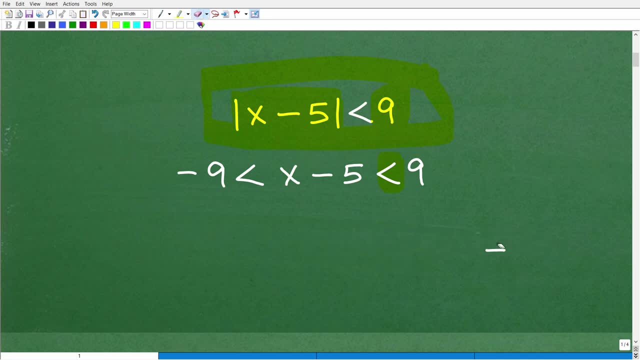 OK. So again, these problems are a little bit more challenging. I'm going to give you some suggestions on how to continue to practice this, But let's get into it. Let's get into this now, All right. So if you understand the setup, OK. what we want to do is kind of like, solve for X in the middle. 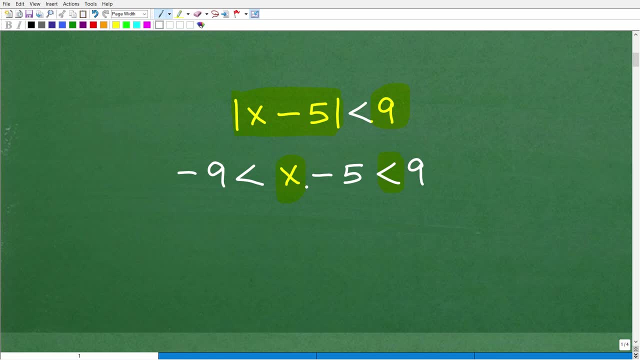 And this is a compound inequality here. So to get X by itself, I have X minus five. So I'm going to add five to everything. OK, Again, this is how you solve a compound inequality. So I have negative. nine plus five is what, That's four. 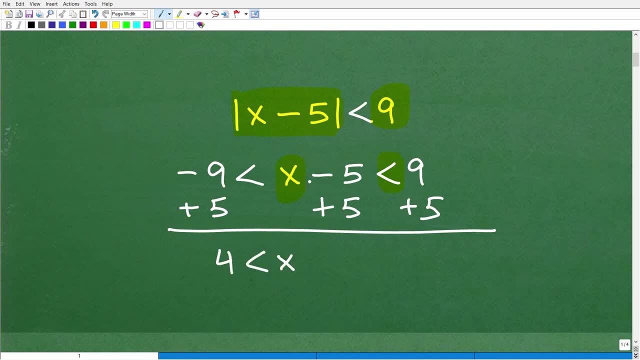 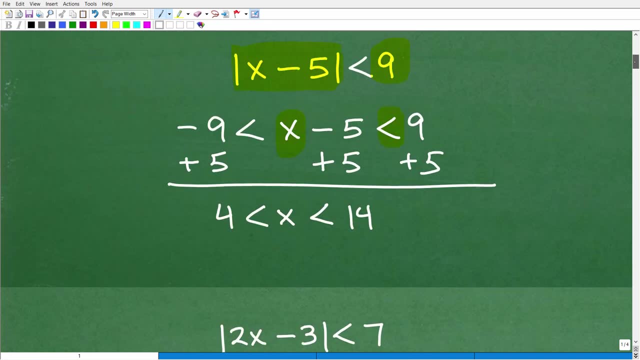 OK, And this is going to be less than X. All right, The fives go away is less than 14.. OK, So that's another problem right there. But let me go and scoot this down and give ourselves a little bit more well. 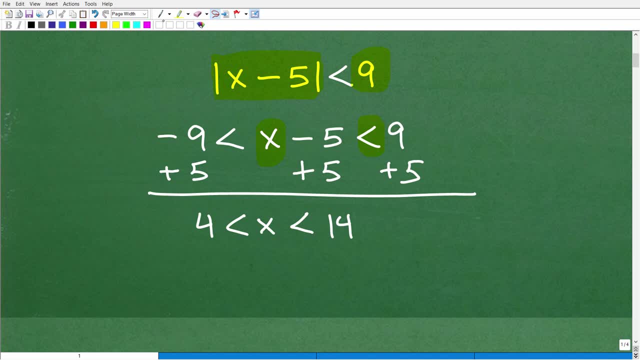 I actually can't do that. Let me scoot it up. Isn't it really cool what I can do with this computer? All right, So anyways. So this is the solution to this absolute value inequality. OK, it's all. X is greater than four and less than 14.. And then we can graphically show this: 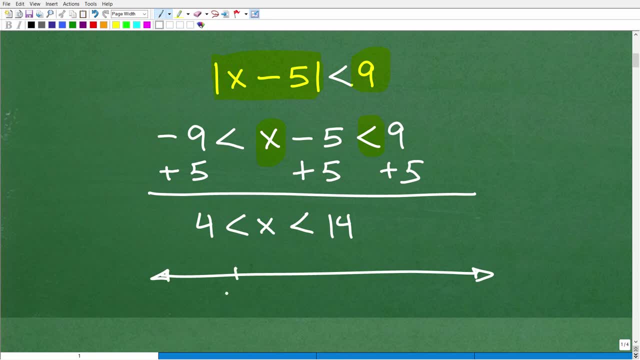 by making a little number line. We'll put our two numbers here, 4 and 14.. And the way you want to do this is just put two circles here Now, because this is less than and not less than or equal to. 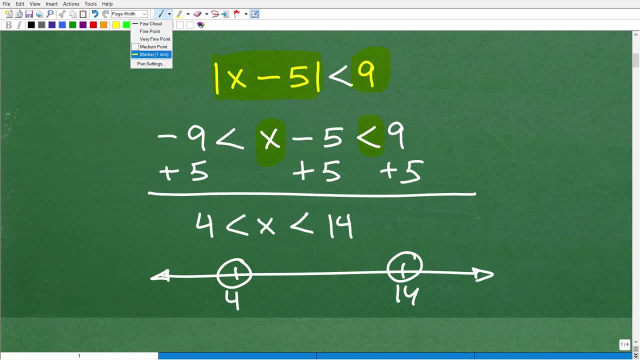 these are going to remain open circles. So all numbers? okay, let's just read this: All x's that are greater than 4 are this way, but at the same time, less than 14.. So this would be the respective graph solution to this absolute value inequality. okay, So you can write it this way, but you also 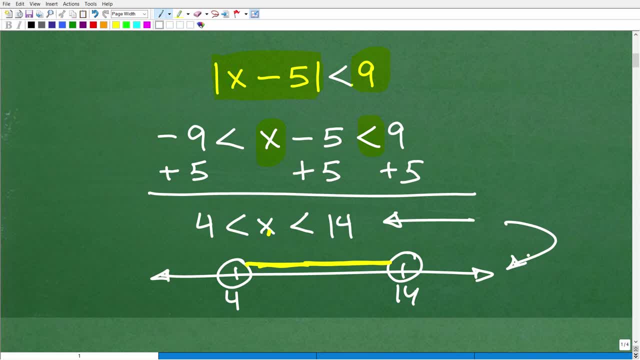 need to understand that you can graph and you'll be required to graph your solutions as well. Again, if you don't understand what I'm doing here, you need to go back and review inequalities, working with linear inequalities and compound inequalities. Okay, so, if this makes sense, well, you pretty much got the main idea, But let's take a look at. 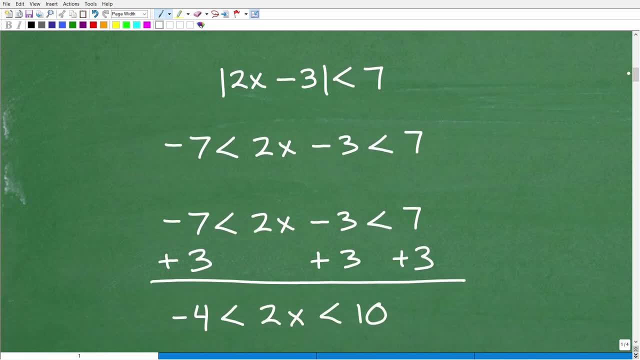 a couple more examples So we can make sure you have this down. Okay, so here we have our absolute value function all by itself on this side, So it's good there- and a number on the other side of the inequality. So we're ready to set this up. So the first thing is we're going to take what's inside. 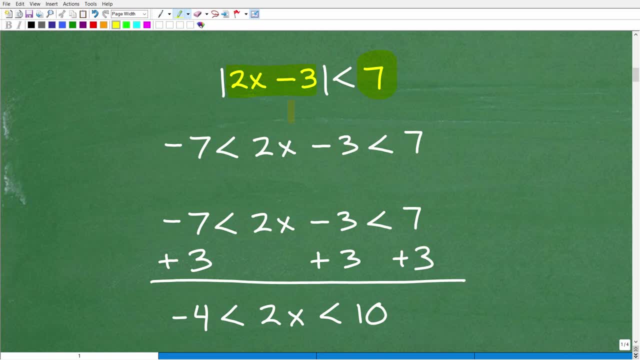 Remember, you drop the absolute value function when you do this setup. It's just what's inside the absolute value function. In this case, it's 2x minus 3.. I'm going to put that in the middle. I'm going to keep my less than. 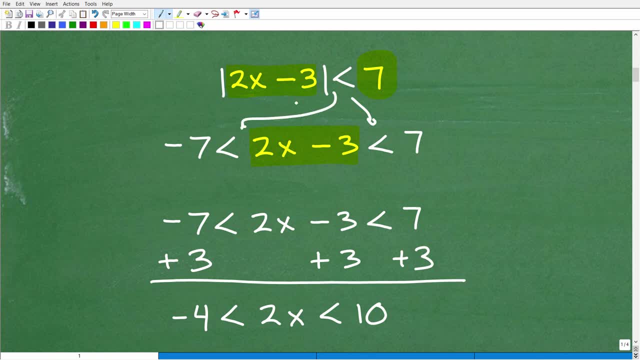 Here I'm going to surround that by the same sign. whatever it is, I'm just going to write it twice. Okay, don't flip it around. Keep that as less than, And then here is going to be the number itself, And then this is going to be the negative of that number, Of course. 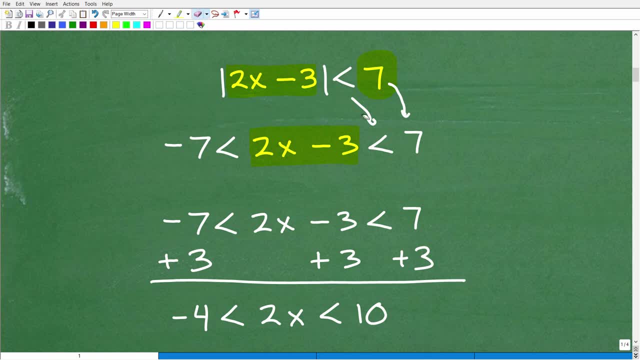 this would be 7 and negative 7.. Okay, so this is the confusing part for a lot of students, is this setup. But once you have this setup, now we just need to go ahead and get this x solve for this x in the middle, ie solve this compound inequality. 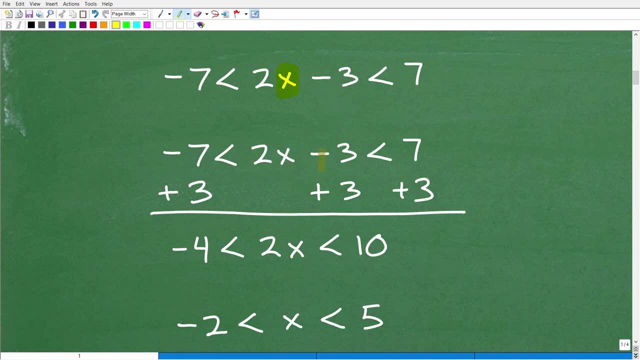 All right, so let's go ahead and take a look at how I'm going to do that. So I have 2x minus 3.. So I'm going to add 3 to everything. Again, if you're confused about this, you need to review compound. 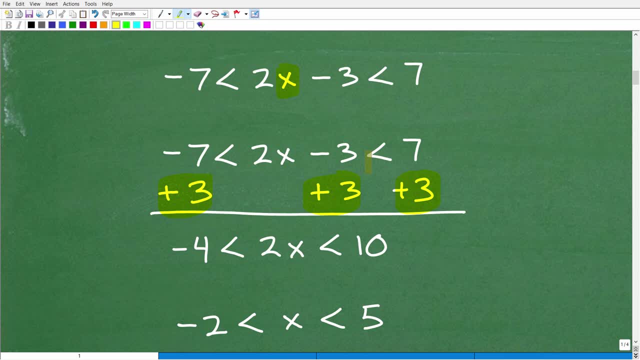 inequalities. That's a kind of prerequisite before you get into this. So I have negative 7 plus 3.. That gives me negative 4.. 2x minus 3 plus 3. That gives me down to 2x. So this is like kind of. 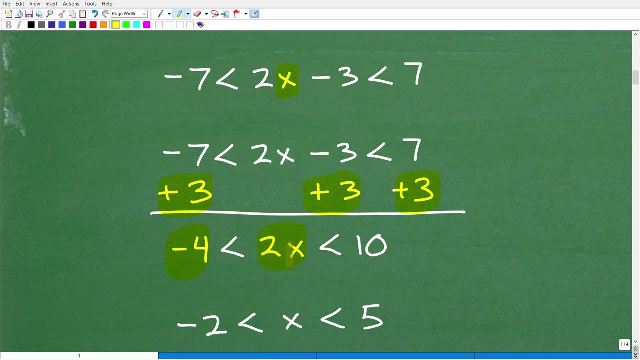 solving for an equation with x in the middle. I'm trying to get x in the middle. ie, that's what I'm trying to do. It's not in the equation, but you're basically taking similar steps as if you were solving an. 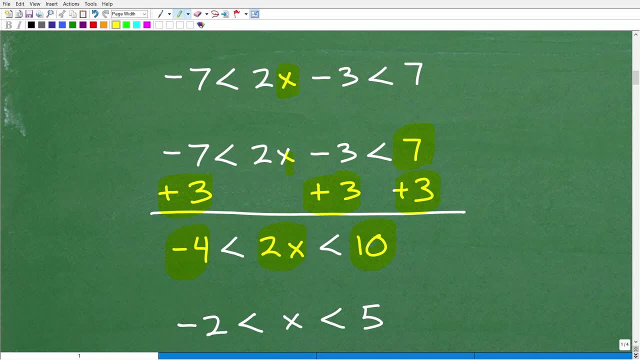 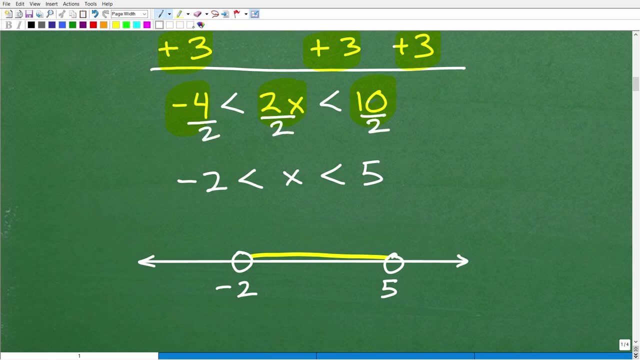 equation. So I have 7 plus 3. That is 10.. So to get x by itself, I'm going to go ahead and divide everything by 2.. Okay, and when I do that, I get negative. 4 divided by 2 is negative, Negative 4. 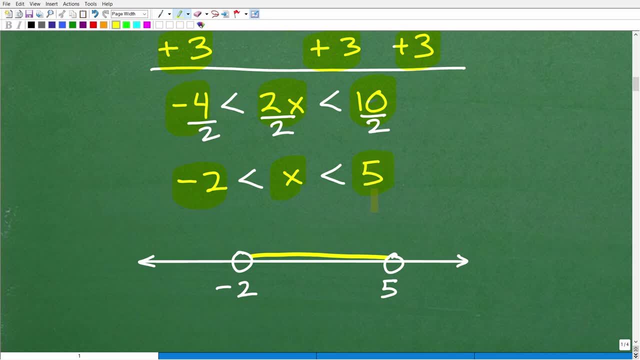 divided by 2 is negative 2.. I get x, and then here I get 5.. And this is the solution. Okay, so what am I going to do? Well, let's go ahead and graph this, because, again, this is very important. What this is saying, this is a compound inequality. I want all. 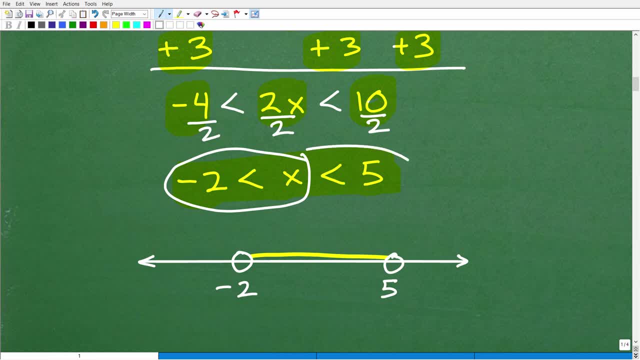 x's all numbers that are greater than negative 2, but at the same time less than negative 5.. So I put negative 2 and 5 on my number line. Okay, remember, negative 2 is over here, 5 is over here and all numbers in between those, negative 2 and 5, are the solution. Okay. 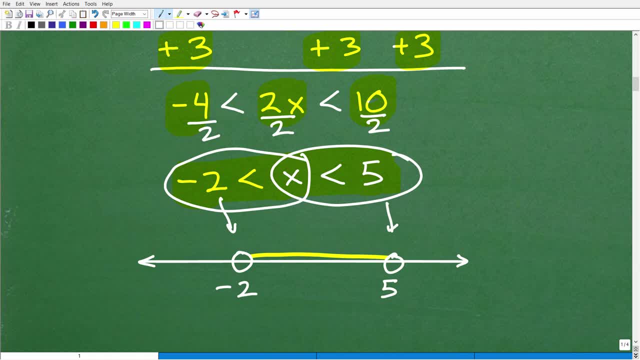 not including negative 2 and 5.. Okay, so we'll see this. We'll see another example of less than or equal to, or greater than or equal to here in a second, where you got to shade these circles in, But these circles are specifically left open. Okay, All right, so hopefully this makes sense to. 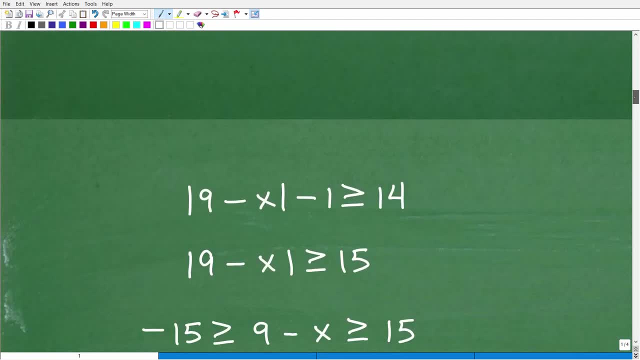 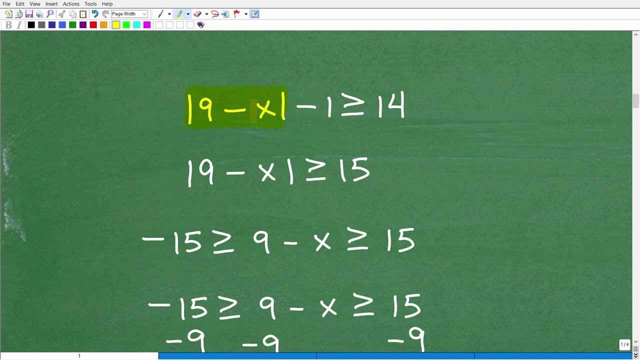 you. And now let's take on a little bit more interesting problem. Okay, so this problem- we have our absolute value portion here, but we have the absolute value portion of this problem is right here. Then we have a number, and now this is a greater than Okay, so this is a couple. 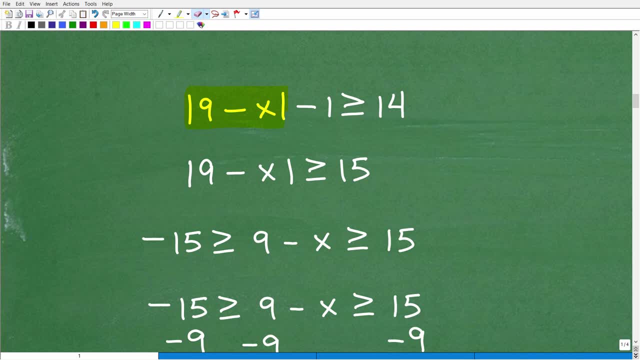 of things. Now, this is, like you know, adding up, or adding a new twist to this problem. So what do we need to do first? Well, the first thing is we want to get the absolute value function by itself on the left hand side and a number on itself on the right hand side. So whatever, basic algebra. 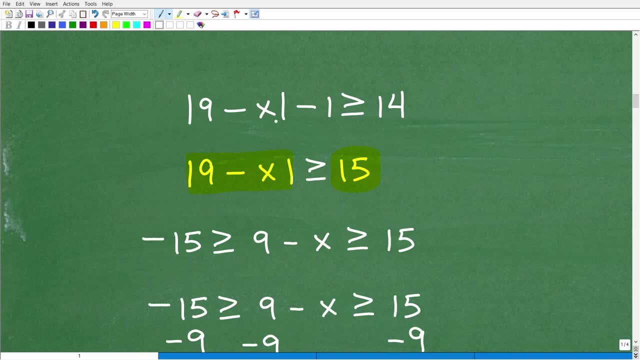 you need to do to get that to look like this? that's what you have to do, Okay, so in this case, I'm just going to add one to both sides of the equation, or sort of both sides of this absolute value inequality. See, I have to be careful, you know, because you know you're doing things that 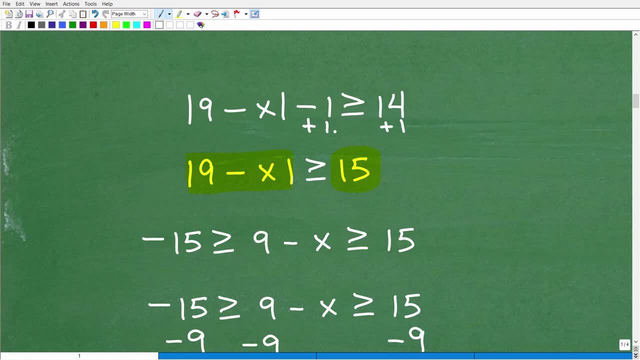 you do when you're solving equations, but this is not an equation. Okay, but you do take similar steps. So here I have: absolute value of nine minus x is greater than or equal to 15.. Okay, so what's the setup? Well, the setup is not going to change. Okay, it's going to be the same concept. 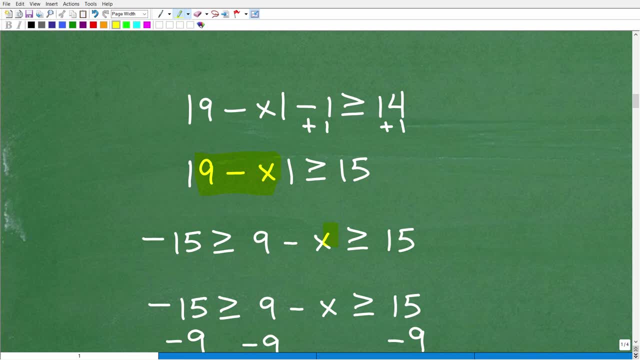 we're going to take what's inside the absolute value function nine minus x. we're going to put that in the middle. Alright, then we're going to put this 15 down here, And then we're going to put this negative of this number, which is going to be negative 15, right here. Again, keeping this is. 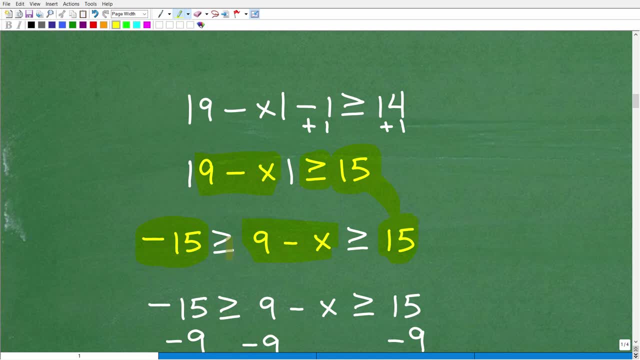 greater than or equal to, right. We're being consistent with that. we're kind of surrounding that nine minus x by this greater than or equal to, just like this. Now I have the work here. Okay, I'm going to show you the full solution. you kind of see what I'm doing, But if you should really 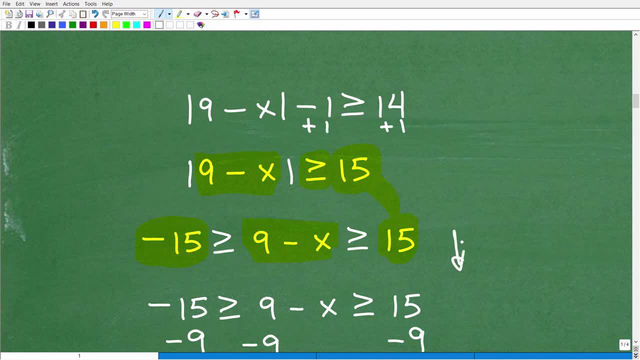 pause the video and see if you can finish this problem out, because that's a good. this would be a good little check to see if you want to do this, So I'm going to go ahead and do that. So Okay, so hopefully you've done that. If you are not ready, go and pause the video, But I'm going to. 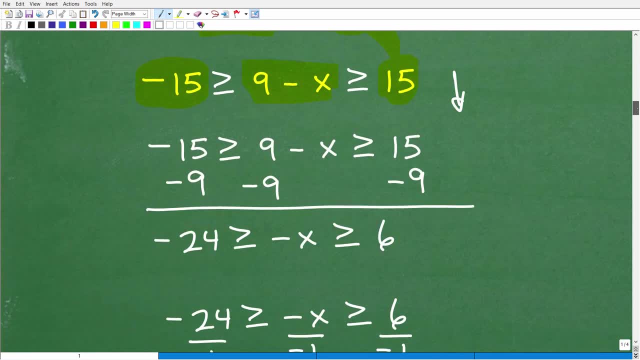 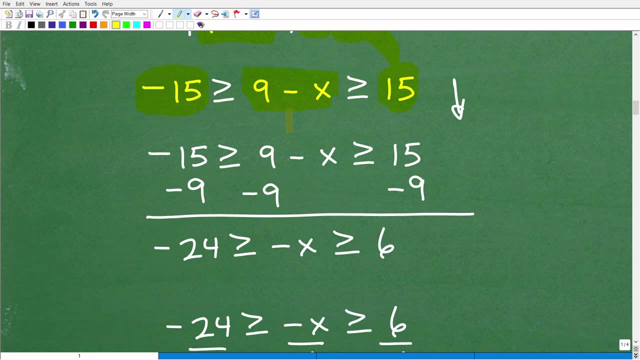 carry on here and finish this problem up. Okay, so how do i get uh x by itself? well, i have nine. i have nine minus x, so let's subtract nine uh from everything here, on all sides of the inequality. so that's going to get my x a little. 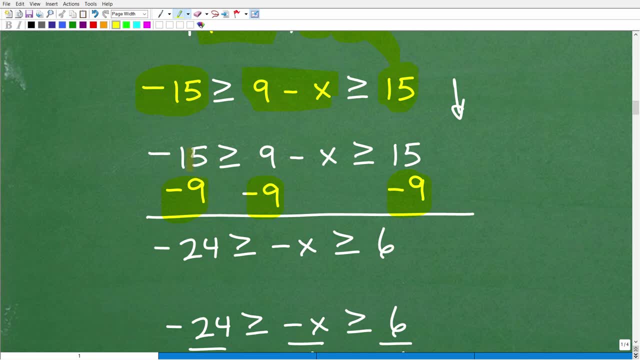 bit closer to me by itself. so when i do this, i'm going to get negative 15 plus negative 9. is negative 24, greater than or equal to negative x. okay, because the nines go away, but i'm still left with this negative x. so that's in the middle, and i have 15 minus 9, which of course is 6.. 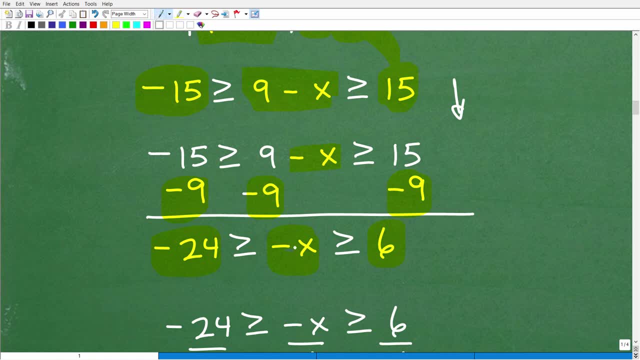 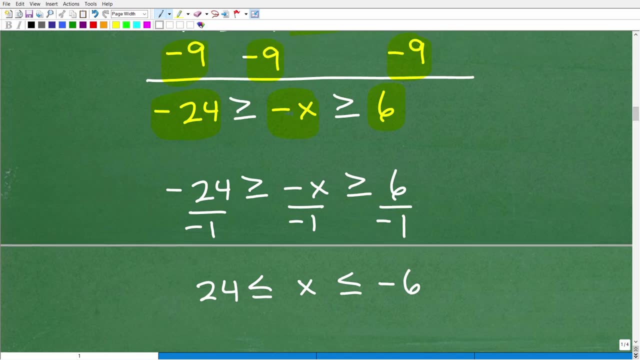 but this is a negative x, not a positive x, so we have to have a positive 1x, okay. so how do i deal with this? well, this is negative 1x, so to get a positive x, i need to divide everything by a negative 1.. now, what happens when you divide by a negative value or multiply by a negative? 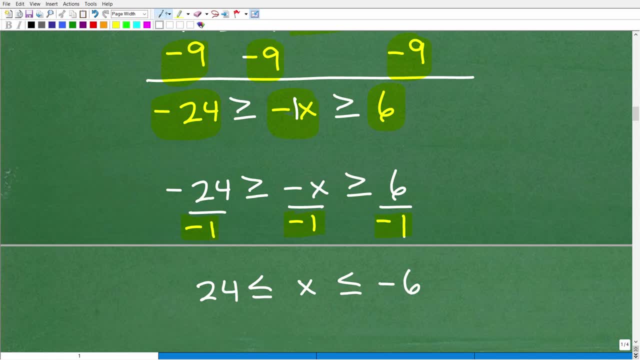 value you on both sides of an inequality. okay, what happens is the um inequality symbols flip. so if you're dealing with a greater than, it's going to go to a less than, and in this case we have a greater than equal to, so it's going to go to a less than or equal to so. 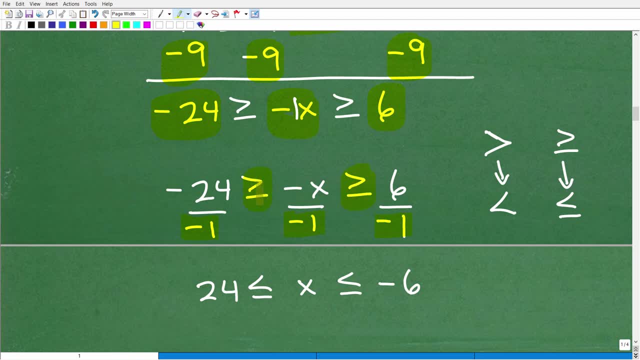 this is a very, very little, subtle detail that if you don't do, you're going to get the problem exactly wrong. okay, so notice, here i'm switching the inequality symbols. okay, again, a prerequisite to do absolute value inequalities is to know how to do linear and compound inequalities. okay, so now. 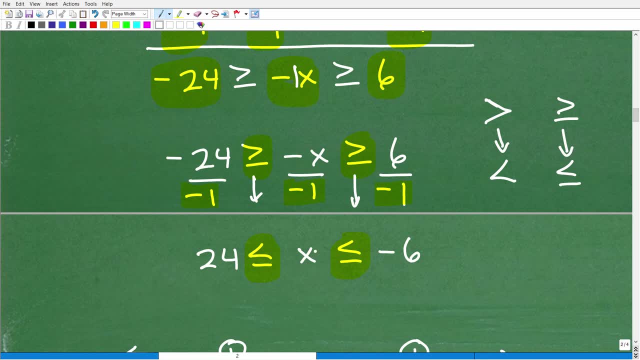 we have x is. let's just read this: okay, we're talking about all x's that are greater than or equal to 24. at the same time, we want all x's that are less than or equal to negative 6.. so what's the graph of this particular in a statement- inequality statement- going to look like? okay, well, 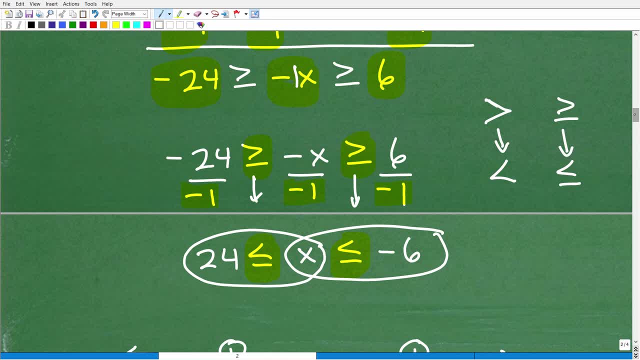 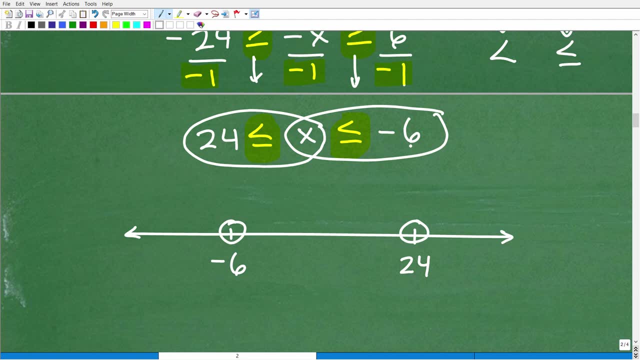 remember, negative 6 is to the left of 24.. and you really got to think about this. okay, so here's negative 6 and here's 24.. just because the 24 is over here and the negative 6 is over here doesn't mean anything. 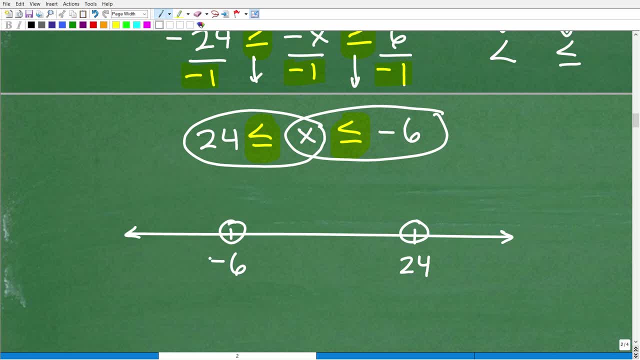 in terms of the graph. let's put these values where they're um at on a number line. okay, all right. so let's read this again. let's start over here. this part of this inequality statement says all x's that are greater than or equal to 24.. where are those x's at? well, they're going to be. 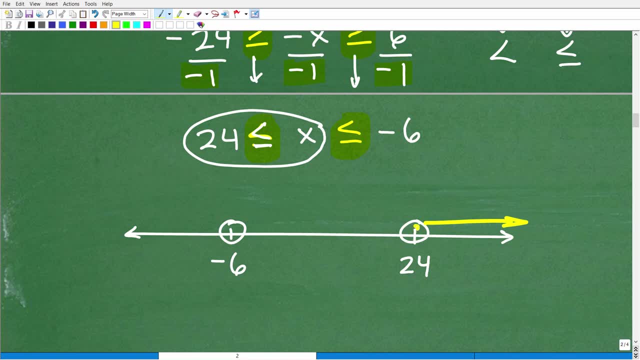 this way. these are all the x's that are greater than now equal to. we have to fill in that circle, okay, so this is very, very important. that means that 24 is in fact. then that number itself is part of the solution set, okay, all right. so now that we have that, let's go ahead and read this: 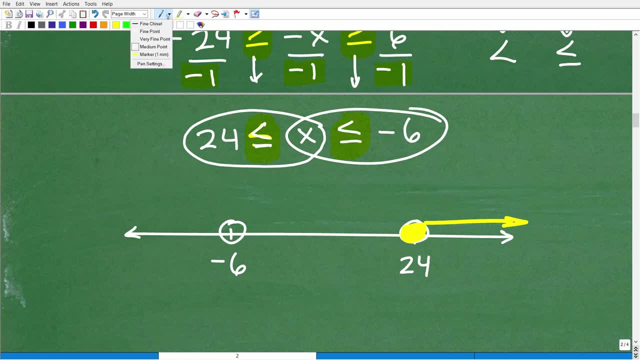 all x's that are less than or equal to negative six are going to be. in what direction? this direction right here. and of course it's going to include negative six, so we're going to fill that in as well. okay, so let's just go ahead and call it a wrap with these. um, couple of problems here there are. 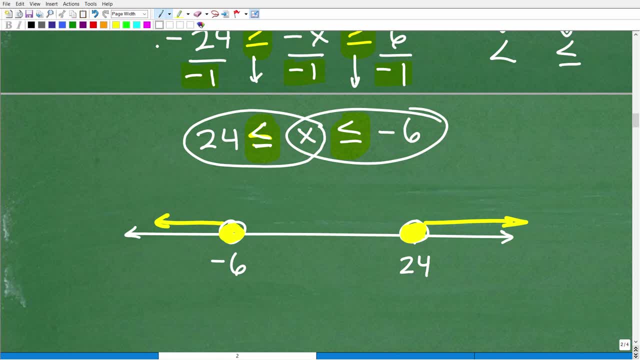 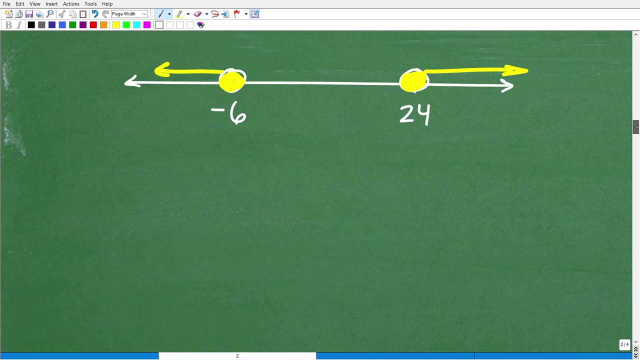 more challenging absolute value, uh, inequality problems. so i'm going to get suggest a couple things to you. one: i'm certain that i've done additional absolute value videos in my pre-algebra and algebra playlist on my youtube channel, because i have over a thousand plus videos on my channel. 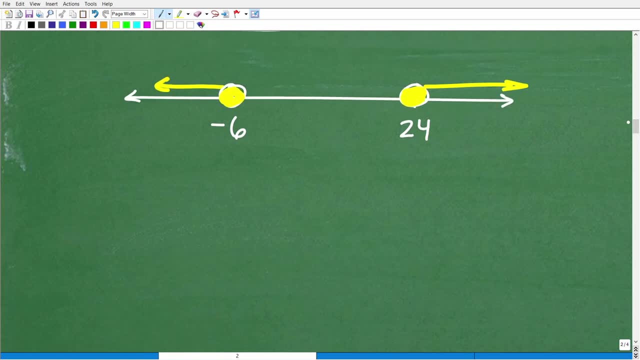 so i may have a ton of content so you can check out some more of my absolute value. uh problems there. but i would highly suggest, if you are really looking to master this, that you check out one of my algebra courses, like my algebra one, algebra two course. but if you know all of this and you got 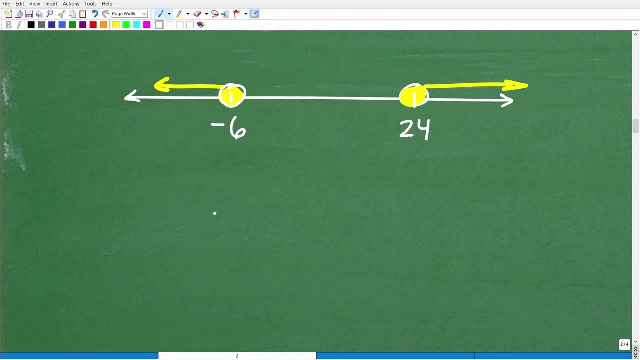 all this right then i must go ahead and give you an awesome happy face. let's go ahead and write it out and let's do the mohawk. today, i'll give you a 1984 mohawk. i think the mohawks were around for. like i don't know, late 70s, 78 and i would say by 80, 88, they were kind of fading out. that was a good thing, but they were pretty cool when they were around, but they just took too much hairspray. so if you're my age, in the 50s, you know exactly what i'm talking about. we used a ton of 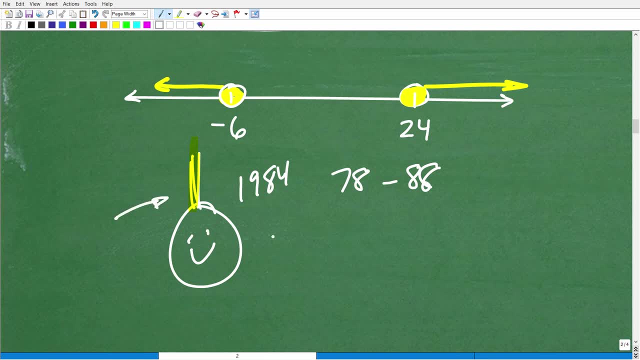 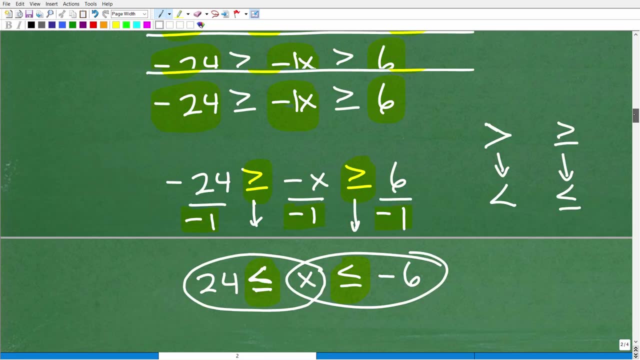 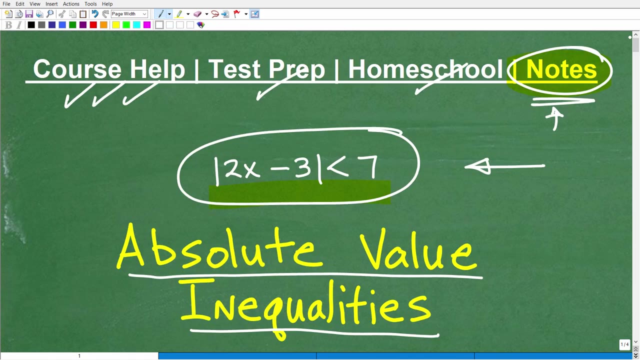 hairspray, but i'm pretty sure our hair was kind of flammable. probably not a good thing, but anyways, let me give you an a plus. any 100 percent nice work, okay, but um, here's the deal. if you didn't understand this, you need to uh to learn this. okay, and probably a couple of uh areas that may be. 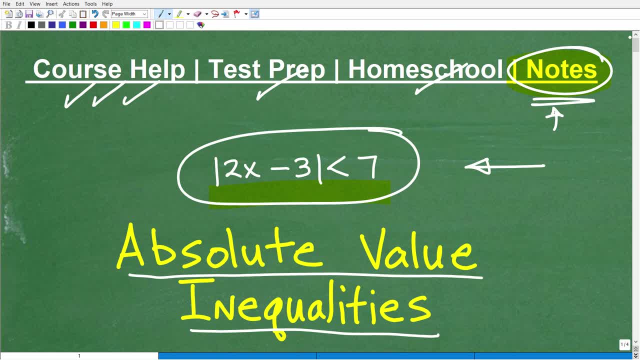 helpful to you is your knowledge of compound inequalities and inequalities in general. so make sure you got that down before you start tackling absolute value inequalities and then don't confuse what you do with the absolute value equation with an absolute value inequalities. that's why note taking and focus is so critical. there's just so much little details that you have to. 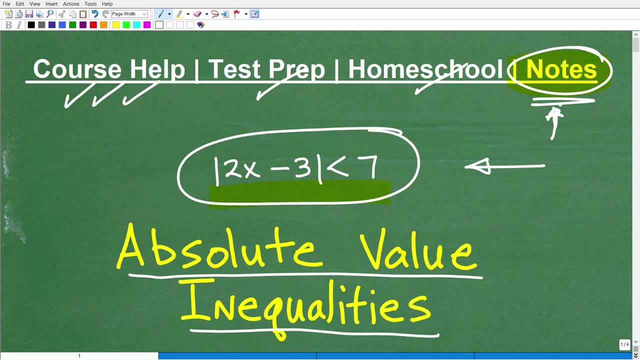 really, you know, be paying attention to in order to get these problems right. but you can get them right. you just got to break all these down in their small little component pieces and hope. this video- uh, hopefully this video- has been helpful to you and i'll see you in the next video. bye, bye, bye. 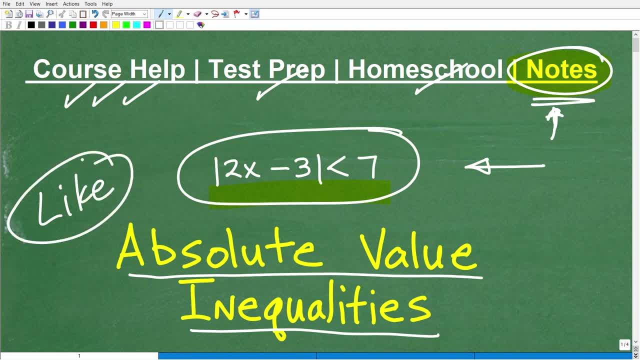 this video helps you out as a quick review, or maybe this is an introduction to absolute value inequalities, but you know you need to carry forward and practice more challenging problems. but anyways, don't forget to smash that like button. that definitely helps me out. and again, uh, if you're new to my youtube channel, uh, please consider subscribing. i've been on youtube for 10. 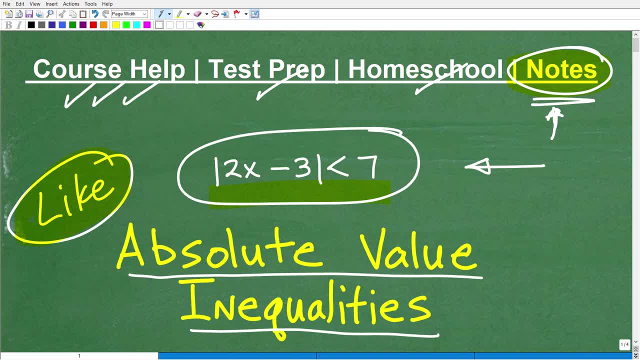 plus years have over a thousand plus math videos, basic math all the way to um calculus. so again, you know my whole you know effort. what i'm very passionate about is trying to really take a step back and do a good job of understanding the problems and the problems that we're facing. 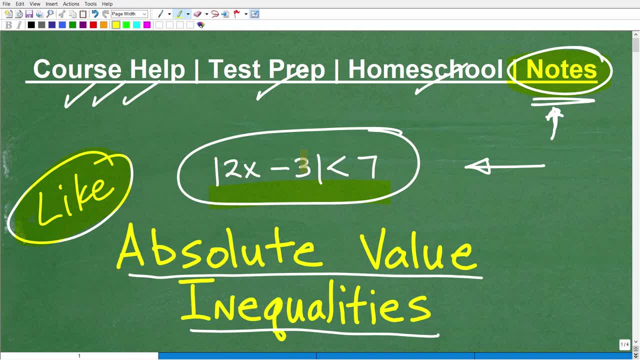 and to really get to a conclusion and to really learn how to do a good job of doing it in a way. that's really important. so i hope you enjoyed this video and i'll see you in the next one. so if you like my content, please- uh, you know- take advantage of all the videos i've posted. 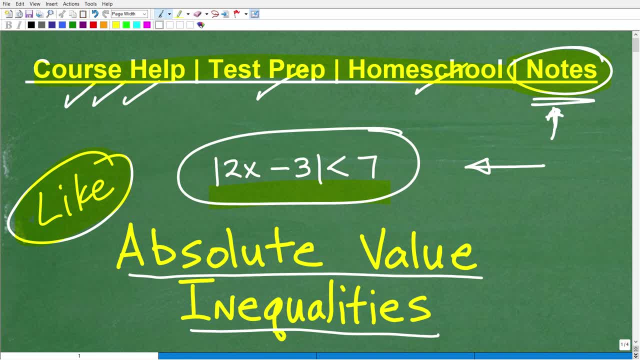 but my best math help will always be within my math help program. okay, so, with that being said, i definitely wish you all the best in your mathematics adventures. thank you for your time and have a great day.